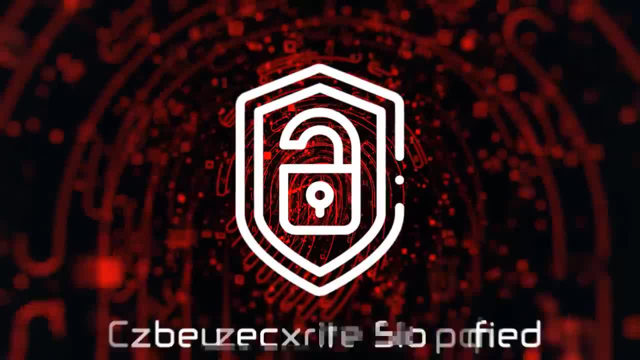 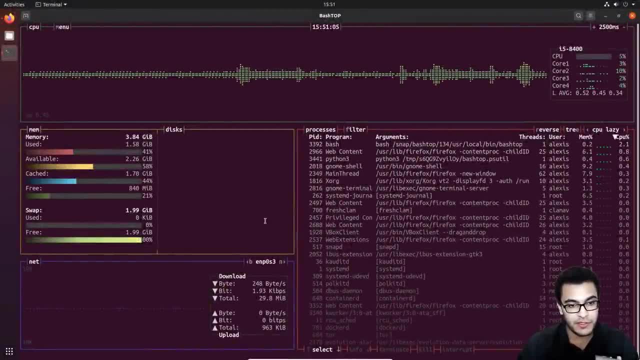 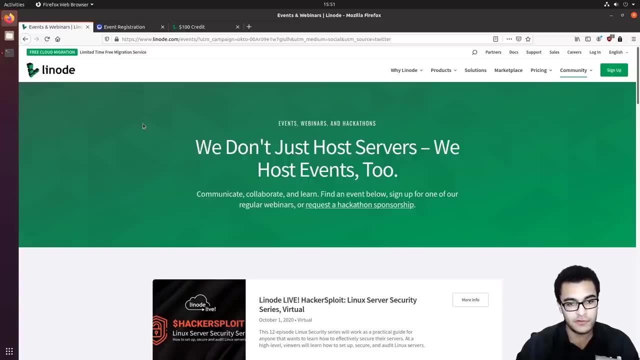 Before we get started with today's video, I just want to take you through the structure of this particular series. So I've actually partnered with Linode to bring you this series. This series will involve two parts, So if you head over to linodecom under events, you should find the Hack. 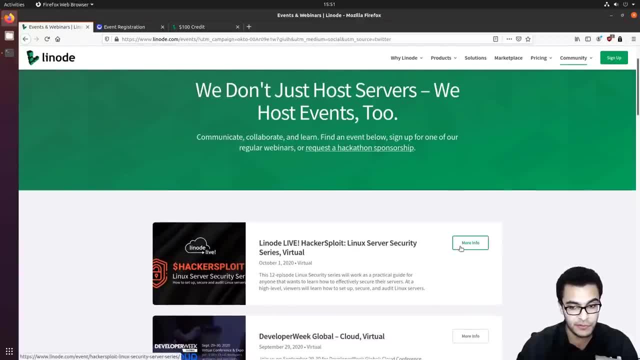 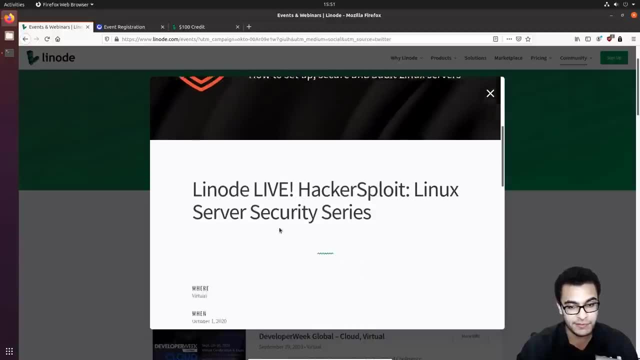 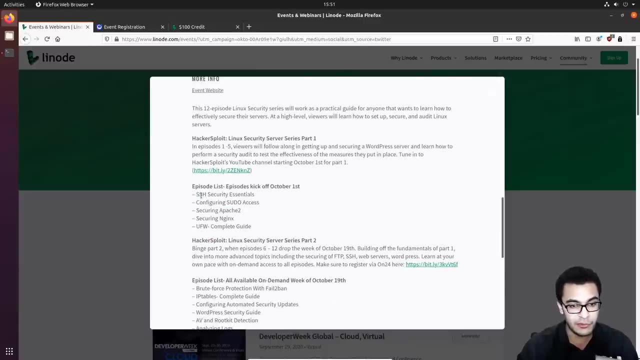 Exploit Linode Live Linux Server Security series and you can just click on more info here. So this series is going to be a 12-part series on how to set up, secure and audit Linux servers and will begin on the 1st of October, And the first series will be available on YouTube and will include SSH. 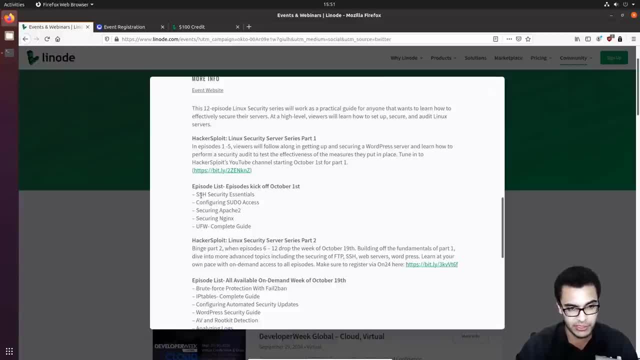 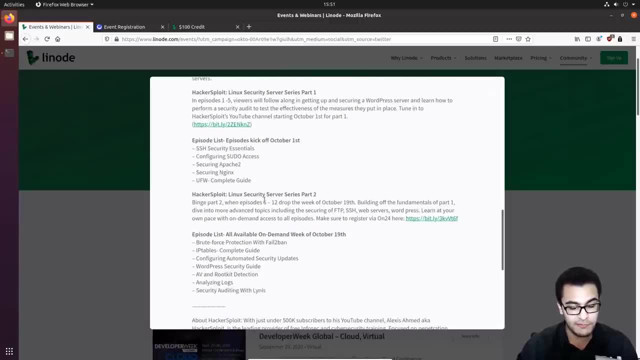 Security Essentials: Configuring Pseudo Access, Securing Apache 2, Securing Nginx and the Uncomplicated Firewall. The second part of the series will be hosted on Linode Live and it's absolutely free. You don't have to pay anything and, again, you can actually register for that. 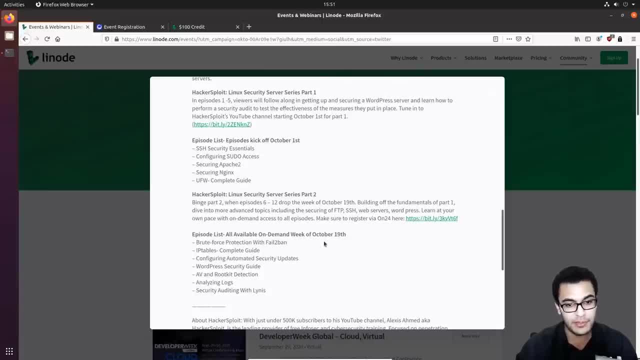 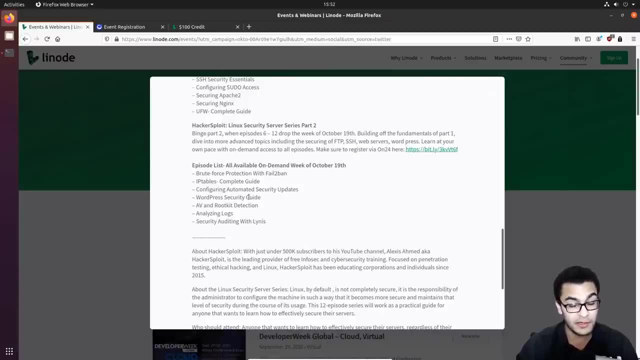 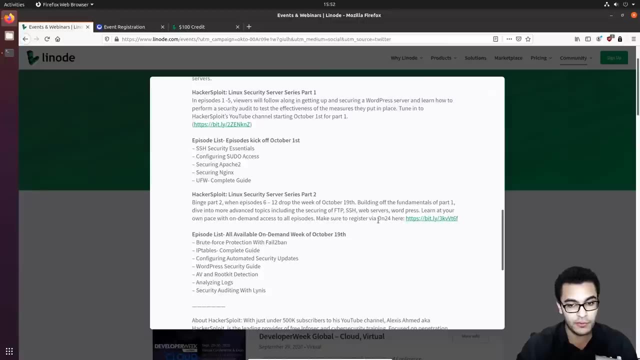 there. This is going to be an advanced series that will build up or build off the first series and will cover things like brute force protection, IP tables, WordPress security and security auditing on Linux with the Linus tool. So to access that, just click on the registration link on the ON24 platform and. 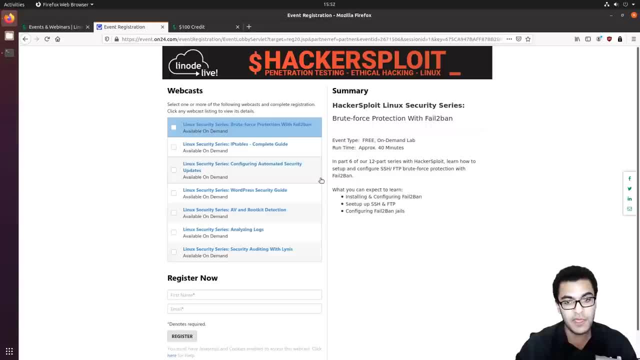 that'll take you here, So that'll give you an idea of all the various webcasts and when they're going to be posted, and it'll give you a summary of what will be covered exactly. These are advanced webcasts that will be about 40 minutes. 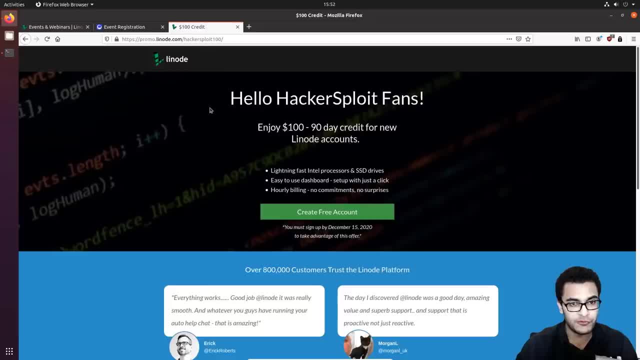 And you can register for them absolutely free of charge. We've also partnered with Linode to give you guys a free credit. So again, if you are interested in using Linode for your virtual private server or for your hosting- whether you're a developer or a administrator- you can get. 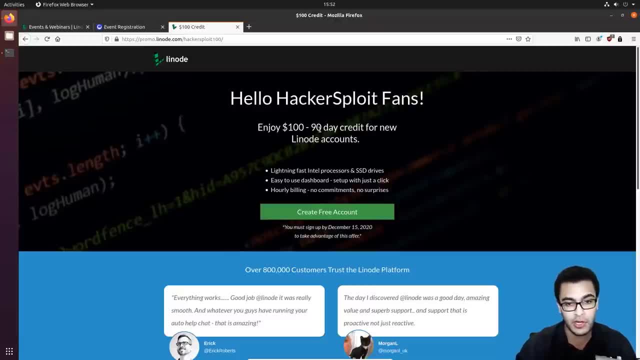 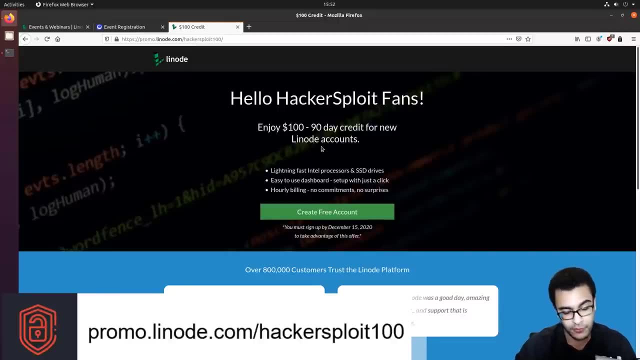 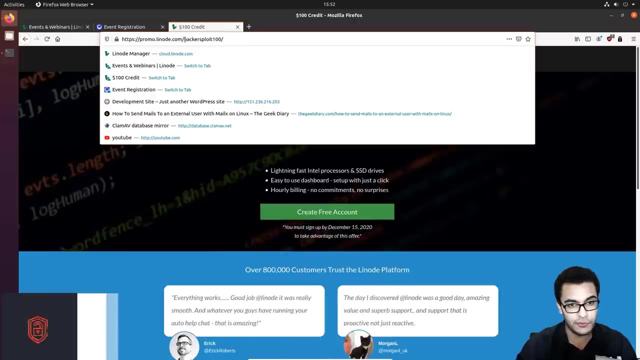 $100 of 90 day credit, And this is for new accounts, So that's fantastic. Definitely do take advantage of this. if you're getting started with Linux or you're actually following, you're following along with this series- You actually redeem this offer or this code, which is under promolinodecom, And the code is: 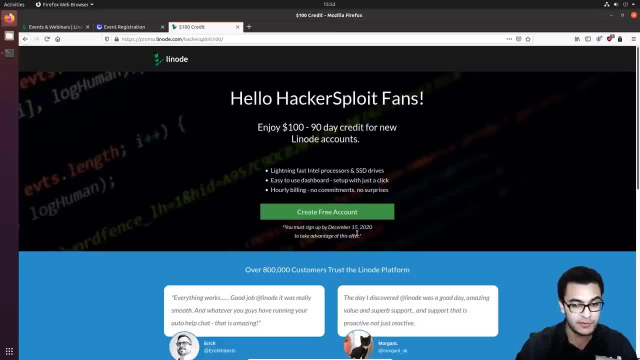 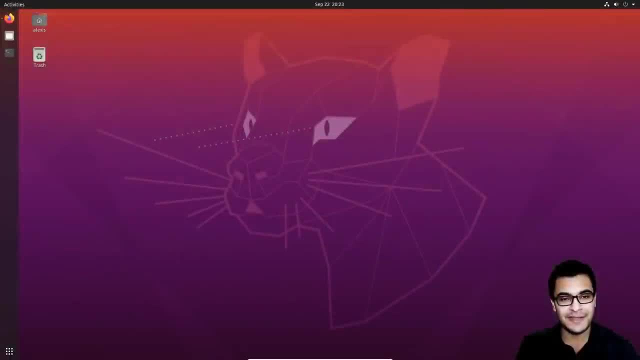 Hackersploit100.. This offer will only be limited till the 15th of December, So definitely check that out. That being said, let's get started with today's video. Hey guys, Hackersploit here back again with another video. Welcome to the Linux security. 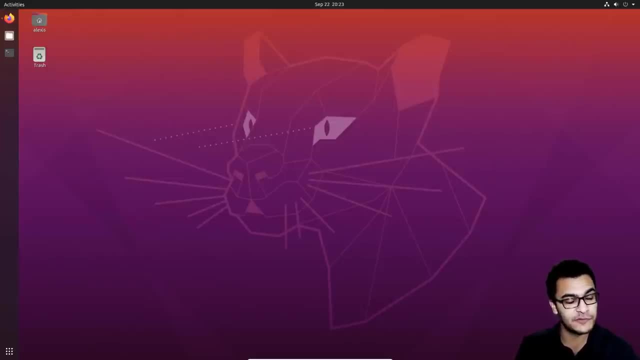 series. In this particular series, we're going to be taking a look at our secure Linux systems and, more specifically, Linux servers. This video is going to be about SSH security, So I'll be taking you through all the essentials of securing SSH. We're not going to be taking a look at brute force protection, where I'm just going to 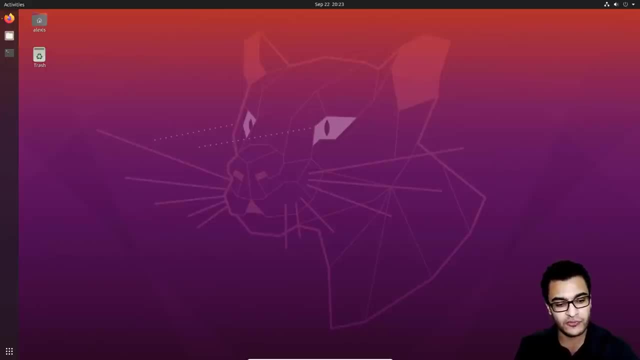 be showing you how to secure SSH and how to go about setting up SSH securely. Now, in this particular video or in this particular series, we'll be following a very important premise here, or an example, if you will, And the reason I'm doing this is to give the videos a bit more context. in 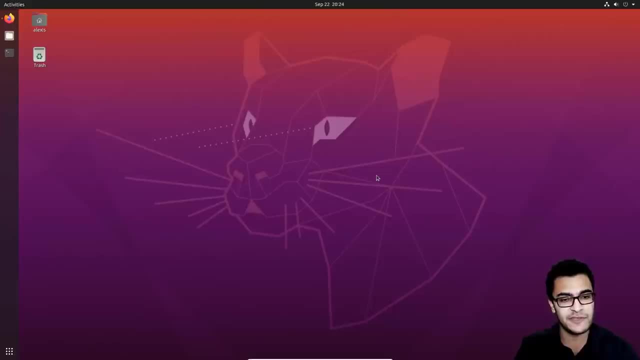 regards to how you can secure SSH. So let's get started. So I'm going to start off by showing you a few tips and tricks that you can apply to secure SSH And, of course, if you are an experienced user, you can take a look at how you can apply these. 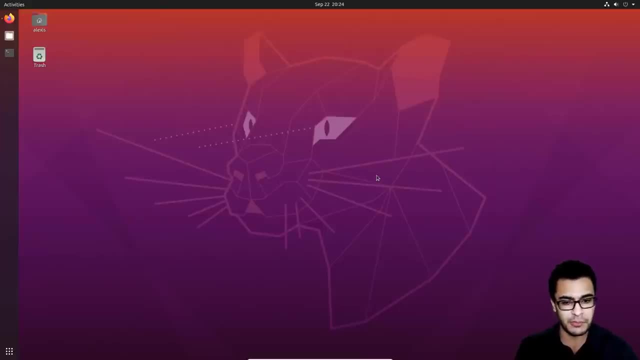 techniques yourself when setting up a server, regardless of whether it's a personal server or whether you're setting up one for your organisation or for your company. it really doesn't matter. So the way I'm going to be doing this is I'm going to be using somewhat intricate but basic 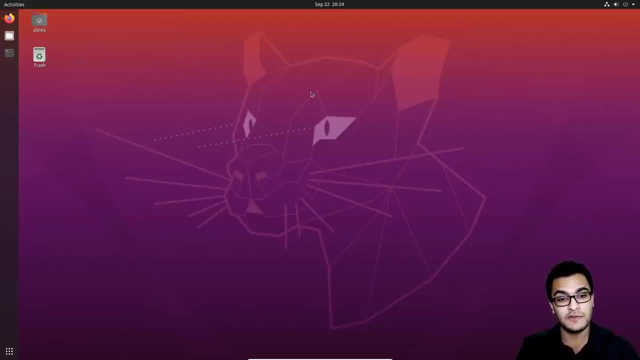 examples again to give you a better idea of of how you can apply these techniques. So in this particular case, we are going to take a simple example of the fact that I'm an administrator and to again manage the company's Linux servers on the cloud and also some various on premises. 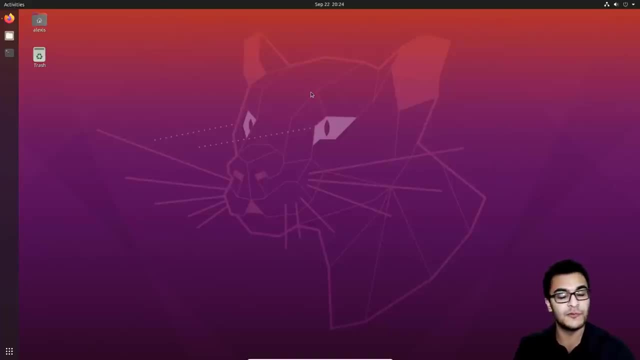 servers that they have And the development team that's responsible for developing the web applications that they have have actually told me the Linux administrator to fire up a few servers on the cloud or virtual private servers for WordPress, for a WordPress website. So we've been 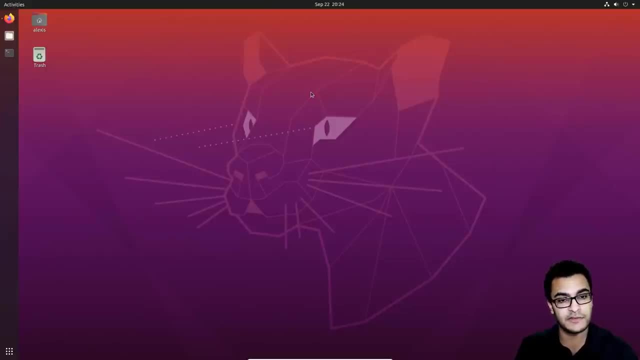 given that that particular role or that particular task, And our first order of business is to set up remote authentication so that the development team can connect to the server and do whatever they want, And of course, they're going to be using SSH to do this. So SSH stands. 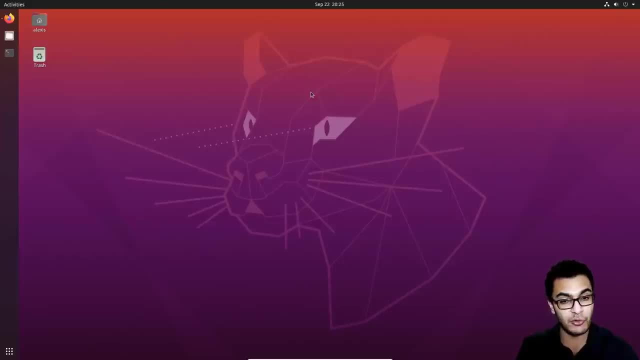 for secure shell. it is a remote authentication and remote control, remote remote control protocol, And it allows you to connect to Linux servers remotely, or even Windows servers Right. so now that we have set up the premise, we can actually get started Now. 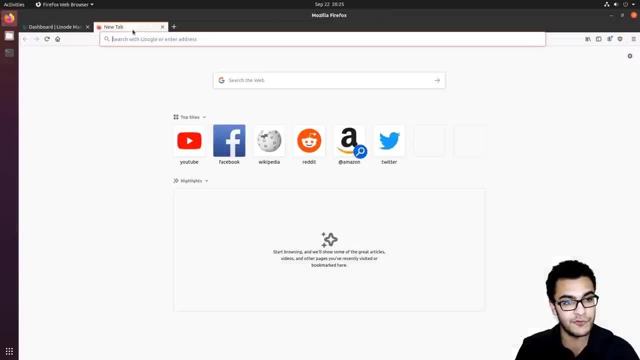 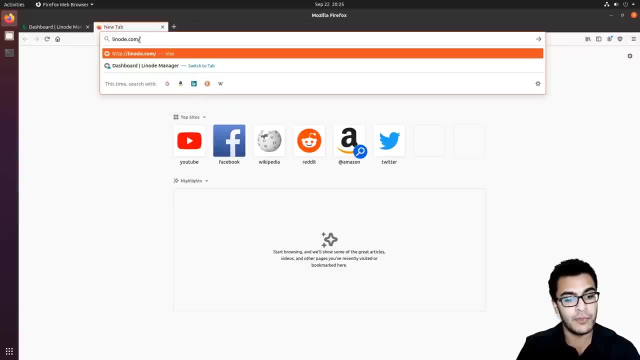 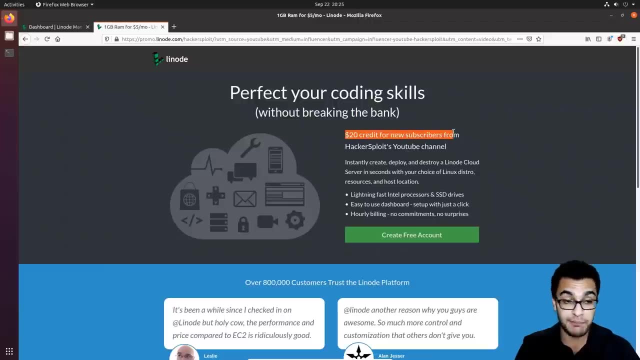 going to go ahead and get started. So we're going to go ahead and get started. So we're going to access- and you can access this by going to linodecom And take a look at hackersploit. So forward, slash hackersploit And that will give you a free $20 credit So you can actually get started. 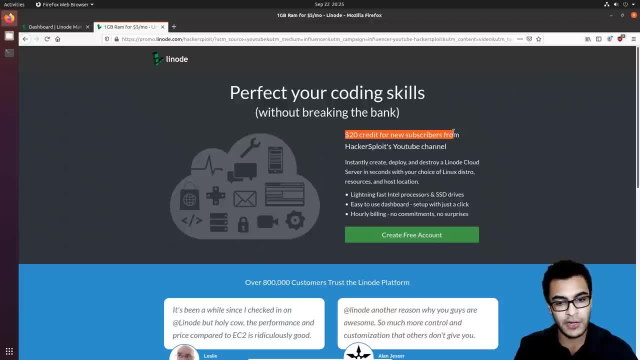 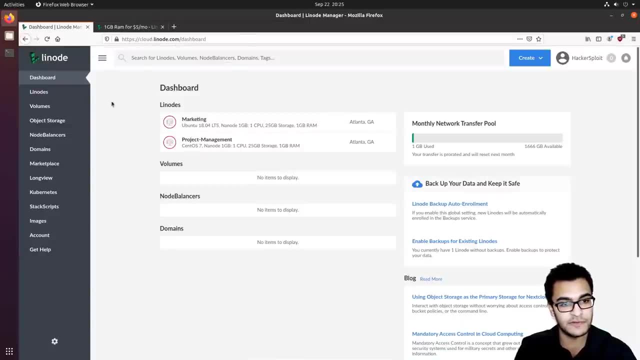 and follow along with this if you want to. And again, you can create as many Linodes as you want and you get about $20, which is fantastic, Excellent. So we can now get started. Now, this is my dashboard And you can see where we are going, or following along with the premise And 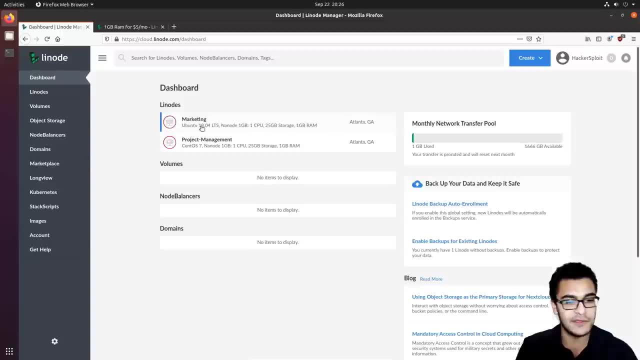 these are the servers that I'm currently managing, And I have the market, the marketing server and a project management server. here And now we've been told to create a new Linux server with WordPress installed and we can go about setting up the security from the. 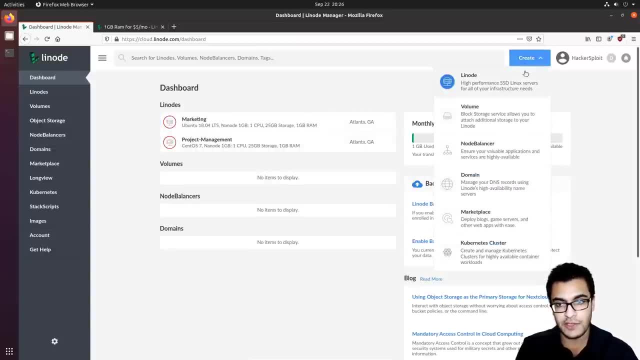 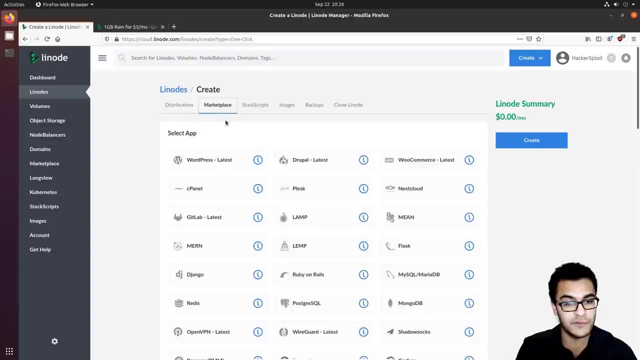 ground up. So the first thing we're going to do is we're going to create a new Linode, So I'll click on new Linode And again, I can set up WordPress manually, or I can go into the marketplace here, which is great, a great feature offered by Linode, And I have all of these applications that. 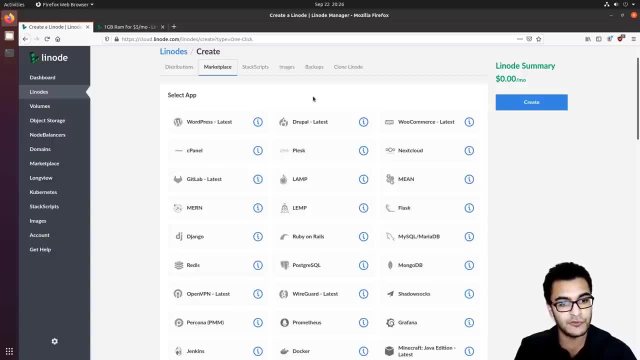 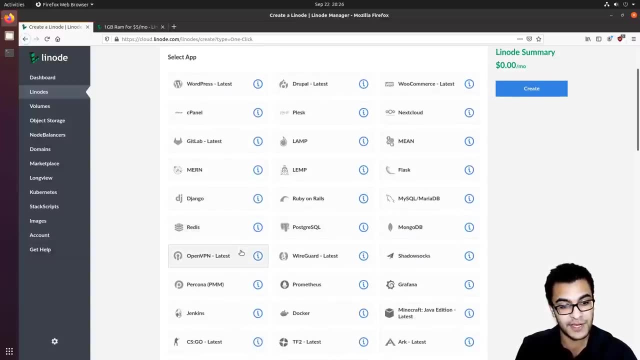 again, are pre configured to work right out of the box, So I can set up a LAMP server, a LEMP server. I can also set up a PostgreSQL database and OpenVPN instance so that I can actually set up my own OpenVPN server. And then, of course, we have the 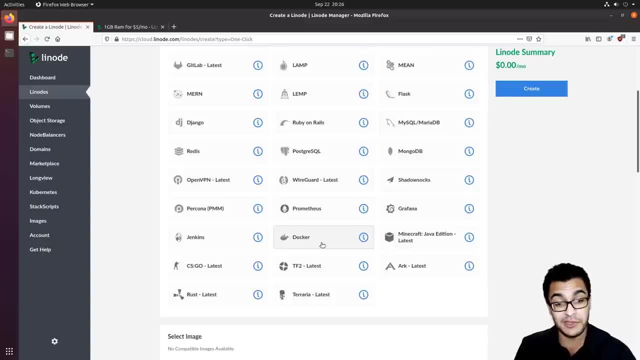 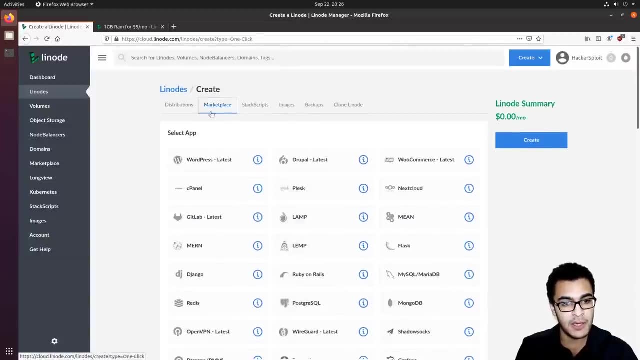 game servers, which is awesome We have. we also have the ability to set up Docker, which is fantastic. you can actually just get started immediately without setting up or installing anything. In our case, we're going for WordPress, So I'm just going to go to. the bottom is going to. 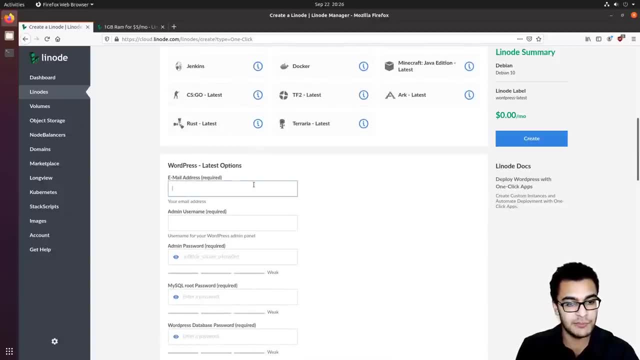 ask us for the WordPress options. So again, the development team is has given us some, some basic credentials And of course we're just going to, we're going to improvise a little bit. So the user is going to be user at testcom And the admin username is going to be admin And of 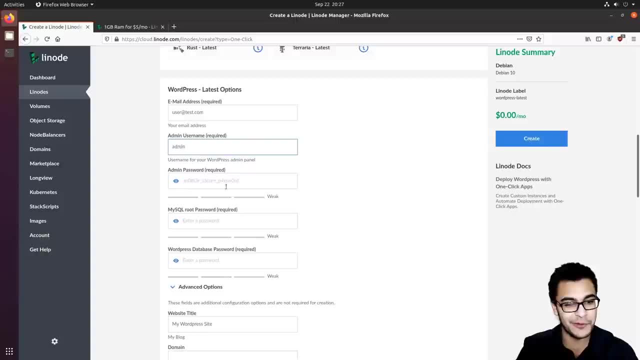 course I don't recommend doing that, But that's another topic for another video. And then, of course, for the password. we're going to give it a super secure password, right? So I'll give it the best password I can And we're going to disable this gradually as we, as we move along, because 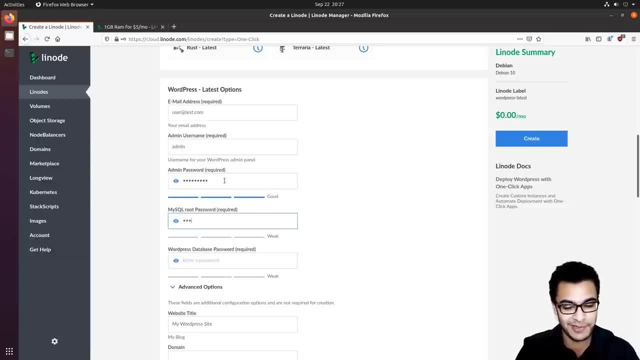 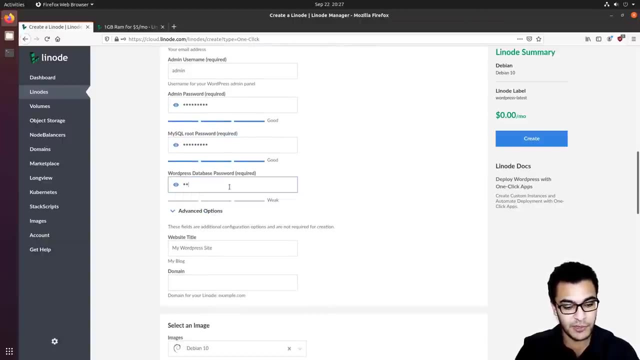 password based authentication with SSH is not really recommended Because you know attackers can brute force the server or brute force SSH. we then need to provide a database password which again make sure that is equally as secure, And Linode gives you a password. 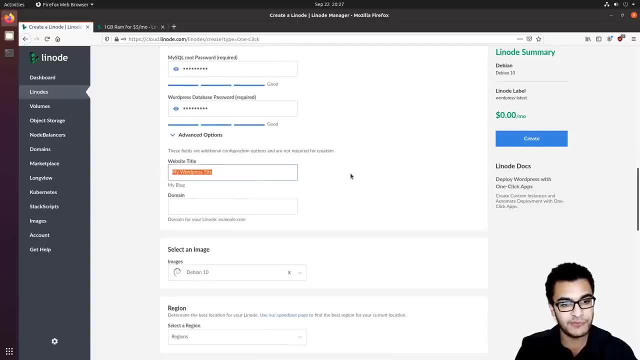 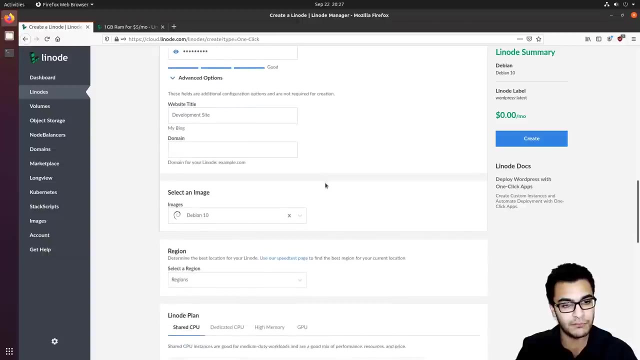 strength level right over here And the website title. we're just going to call this development development site. This is where they're going to. the development team is going to just work on various betas or new, new web apps that they're currently working on And we don't have a 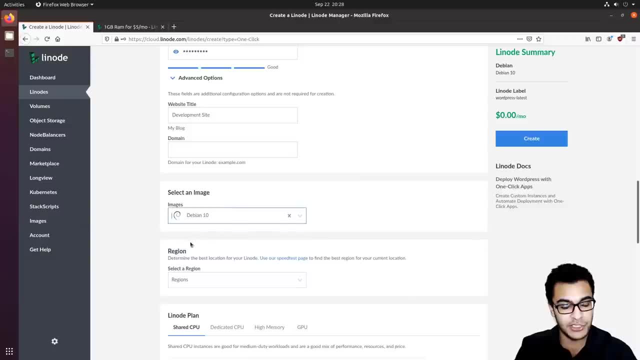 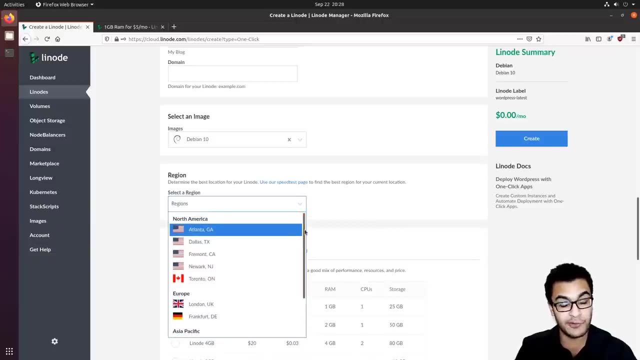 domain yet, So we're not mapping it And the default image is going to be Debian, which is perfectly fine. I then specify the region, And of course, you can specify the region that's most appropriate or advantageous to you, based on what area or what part of the world you're. in my case, 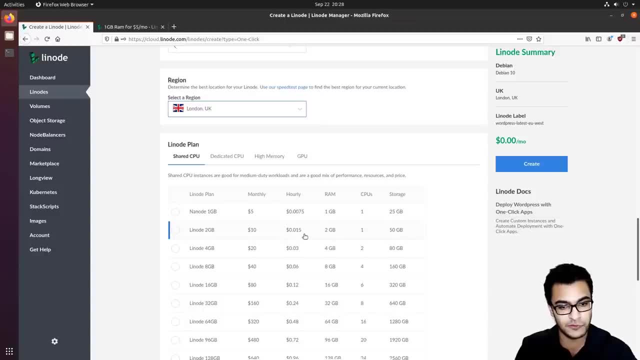 I'll just go for Europe, London, UK, as that's the closest to me, And I can then specify my plan. Of course, these are based on CPU intensive or CPU dedicated CPUs, high memory based, a Linode and a CPU based Linode as well, which is great for password cracking. That's something I'll probably 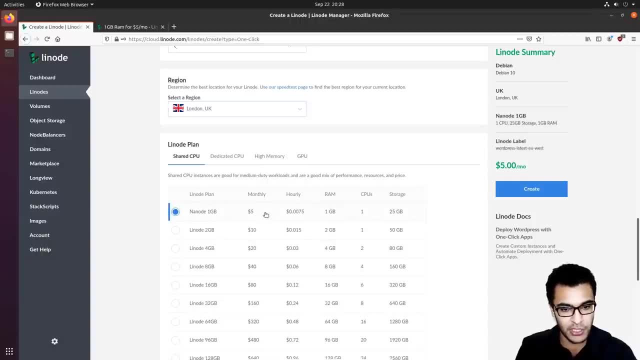 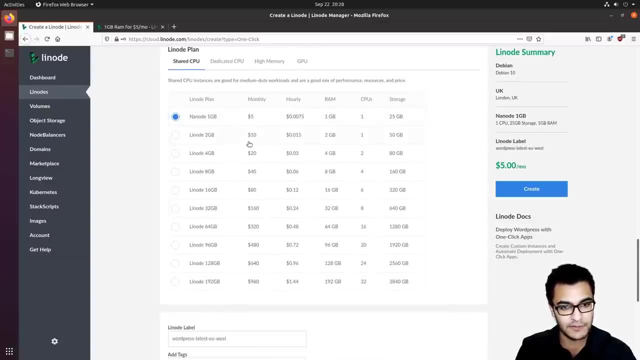 want to cover in another video. So I'll click on a one gigabyte RAM and one gigabyte- sorry, one- CPU Linode, which is a nano, and that's about $5 a month, which is perfect, So that'll be fine. 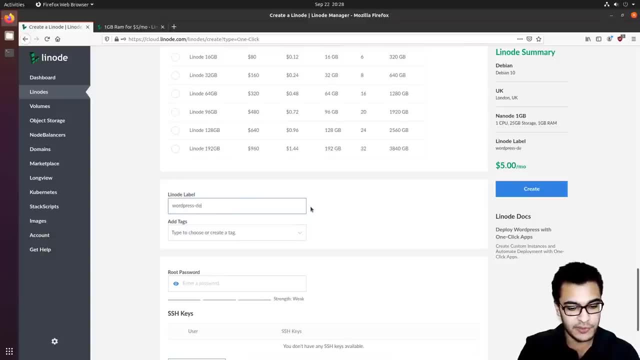 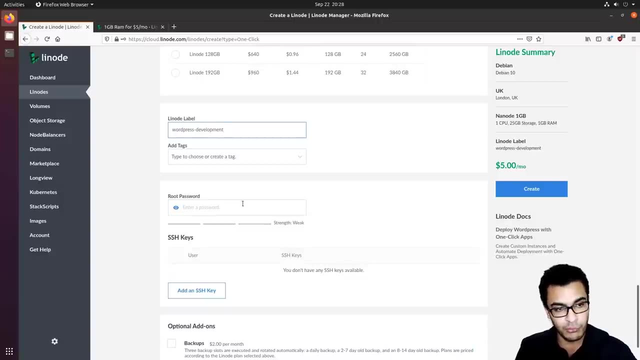 for WordPress server And I'll just call this WordPress development. That's the name of the server, So WordPress development, and I'll enter a root password. Now you can see a very interesting thing here: with most cloud providers, they don't have a root password. they don't have a password. 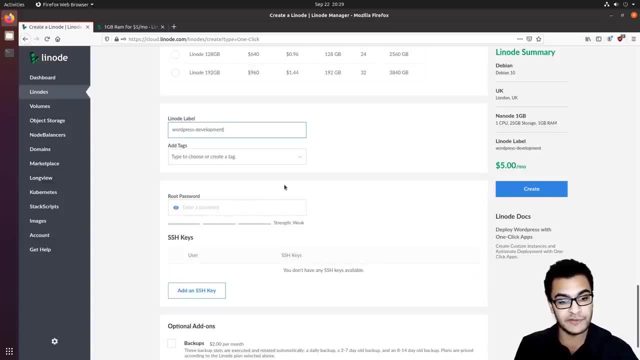 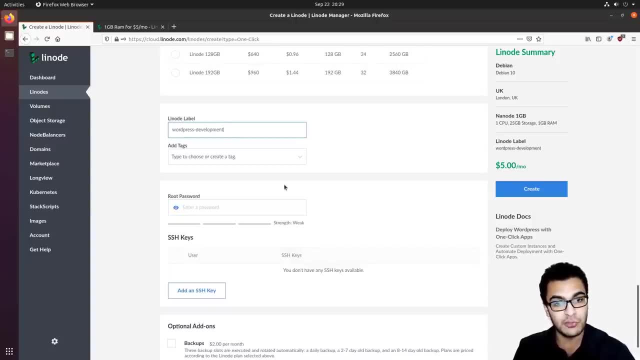 there's a flaw here by default, And that is the fact that you'll be logging in directly to the server with a root user account, which is our first order of business that we want to change. So we'll stick to, you know, authenticating with the password first, and I'll not add an SSH key. 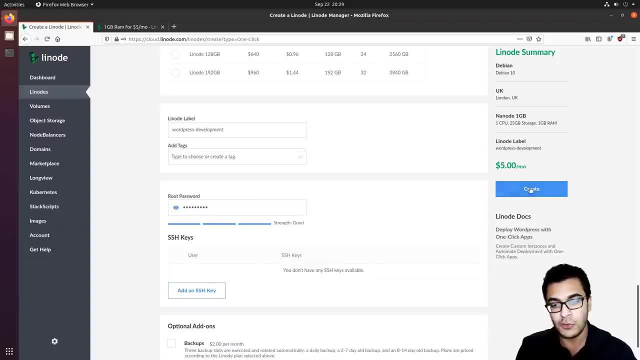 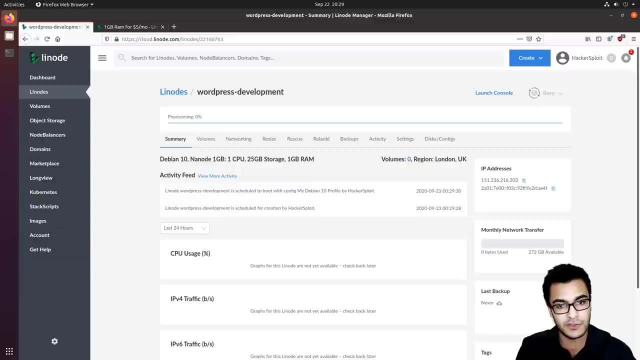 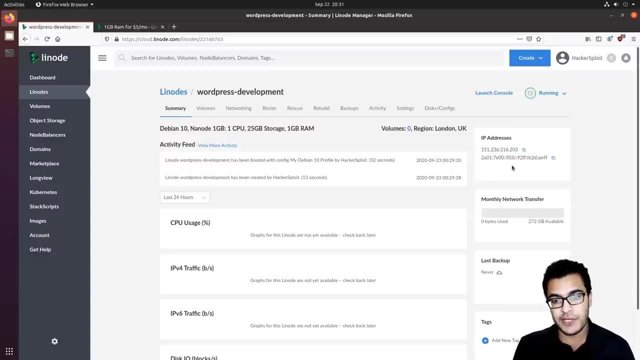 yet, because we're going to add it for a different user. So I'll hit create And that's going to instance for us. So I'll just wait for that to provision and to start And I'll just wait for that to complete. All right, the Linode is created so we can actually get started. So I'm just going. 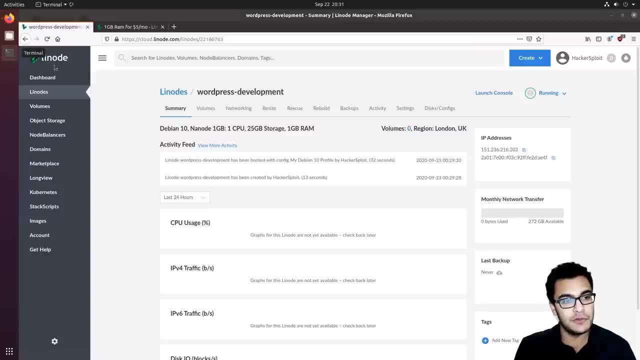 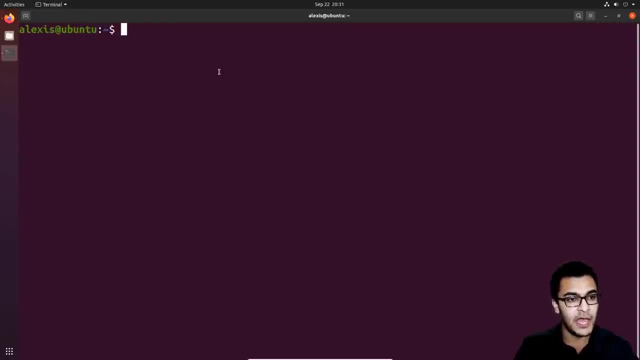 to copy the IPv4 address here And we're going to log in using OpenSSH or the OpenSSH client. Now, as I said, I'm currently using Linux- Ubuntu to be specific- And of course you can log in with various other. you know SSH clients. like you have PuTTY on Windows And of course you have 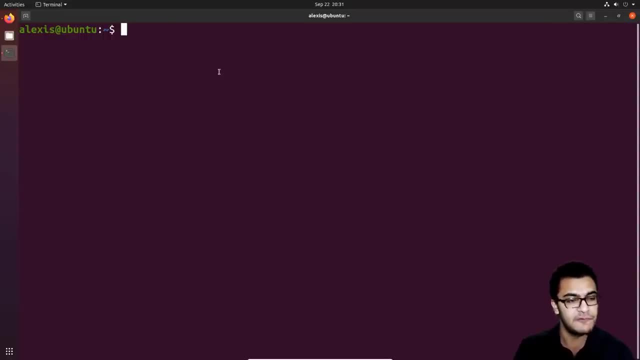 OpenSSH client installed by default on Mac OS, I believe, And on Linux it's pretty much the same. So you want to make sure you have the OpenSSH client installed. So sudo apt install OpenSSH. And we want to specify the OpenSSH client, I believe. There we are And I'll just specify. 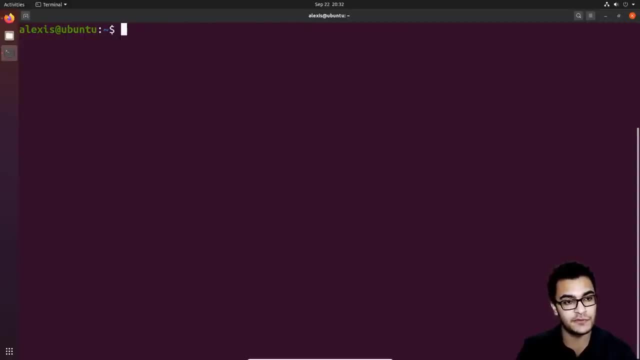 my password here And that's going to tell me it's already installed. Fantastic, So to authenticate via SSH. we say SSH, we specify the username and we'll paste in the IP of the server And then we'll paste in the IP of the server And then we'll paste in the IP of the. 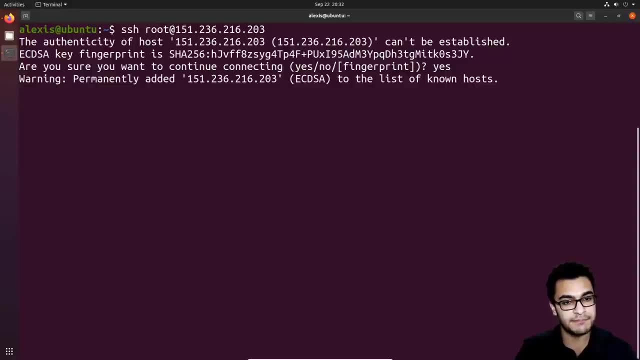 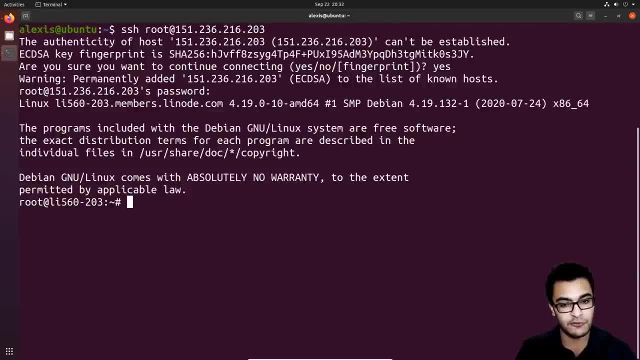 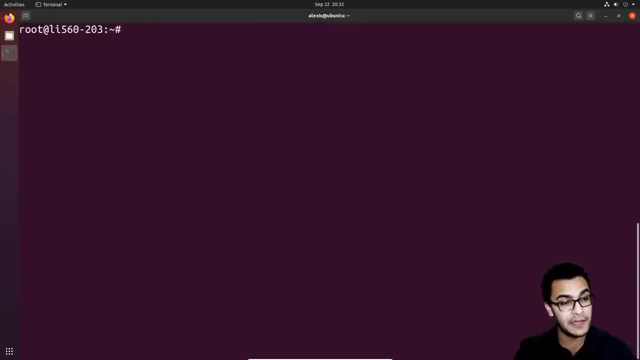 password here And we are logged in- Fantastic. So now that we have access to the server, we can- we can get started with our first, our first priority, which is to add another user, because if I currently list out the users on the system, you can see, apart from the other. 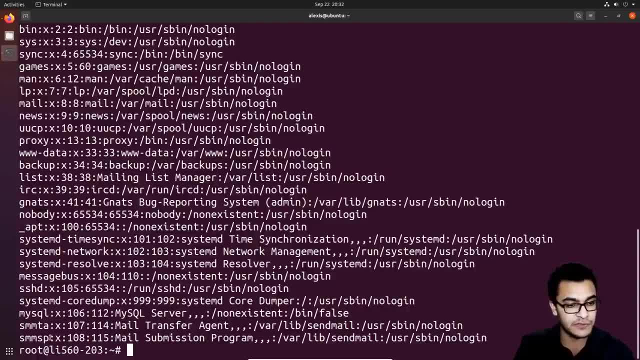 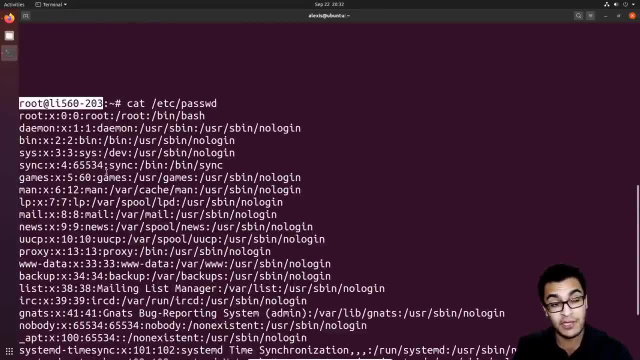 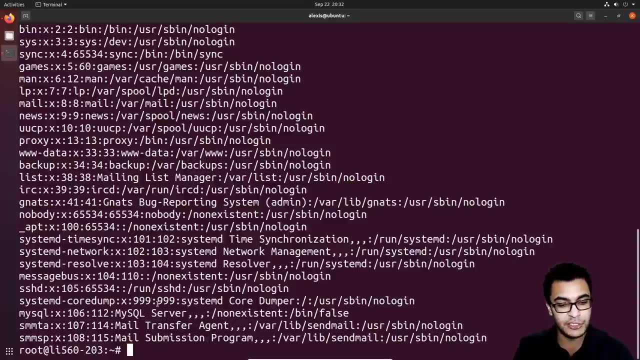 service based user accounts, like MySQL Users, which is for the database And www data. you can see that we only have the root user and we don't have any other user accounts, which is a problem, Because when we talk about the root account and permissions in regards to 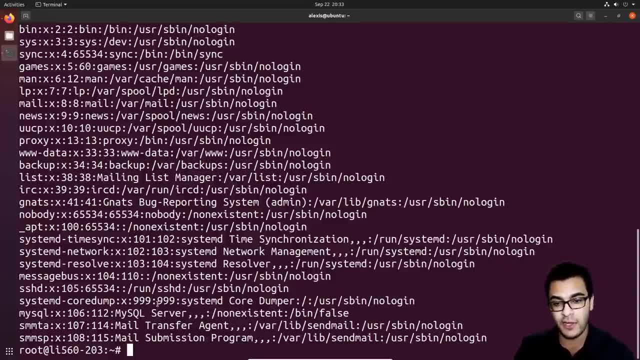 the power of the root account. the root account is like the administrator account, which means you can pretty much do anything, And if an attacker is able to get access to the root account remotely, they can pretty much take over the entire system. they can change passwords for. 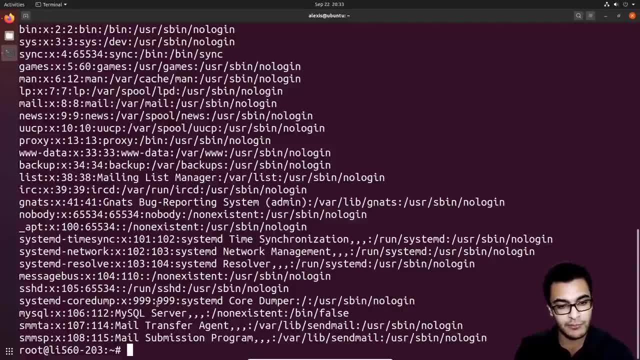 the users. they can. they can, you know, delete databases, dump contents of databases, so on and so forth. So our first order of business is to disable the disable authentication, remote authentication to the server with the root account. And the way we do that is, first of all, 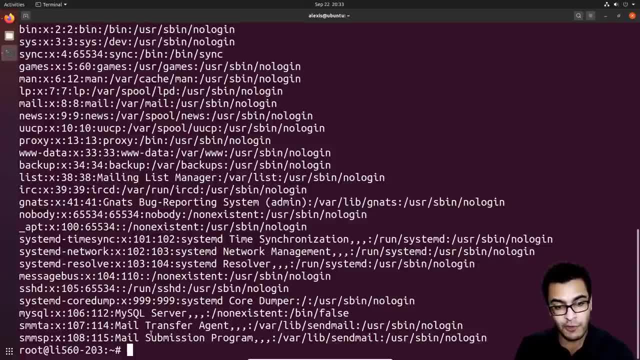 we segregate duties on the server right. So for the development team we'll create a user for them so that they don't have to use the root user to log in. So to do that we use the user add command. So user add. 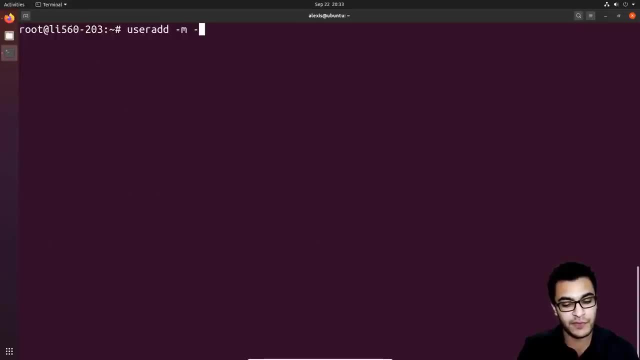 and I'll say M to create a home directory, and we specify the shell, which in this case is going to be bin, bash, right, And. and I'll create the username, which is just going to be dev, and I hit enter. So we've added the user dev And if I just print out the users now, you can see at the 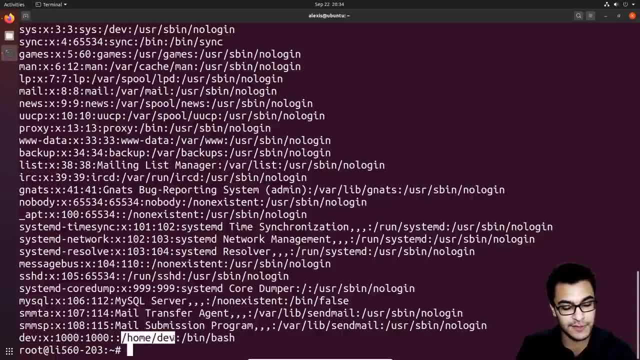 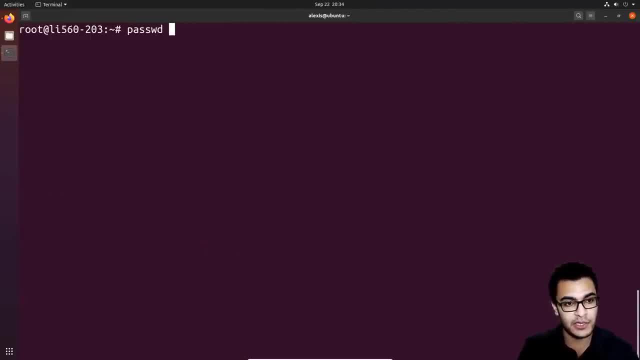 bottom. we have the user dev right over here and the home directory is listed as home dev. So the next thing we want to do is we want to assign a password to the user dev. So I say password and I specify the user dev, So I say password. 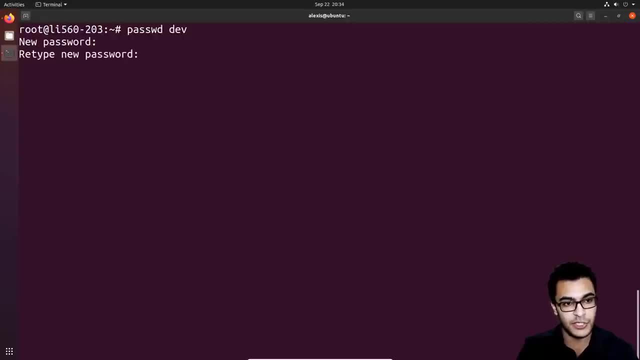 dev. it's going to ask us to specify a password for the user dev, which I will do. And there we are. So we've now added the user dev and we can try and switch to that user by using this super user or switch user that we are. So we say su and we move on to the dev account And you can. 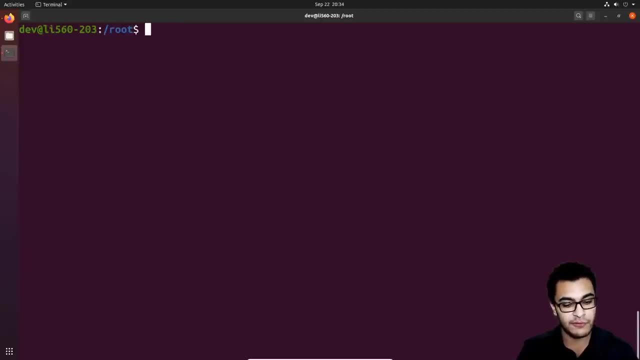 see we can log in directly And if I go to the home directory, you can see we are currently. sorry, TWD, we are currently in the home dev directory here. We can also switch back to the root account, like so, and it's gonna ask us for the root account password, which works out fine So. 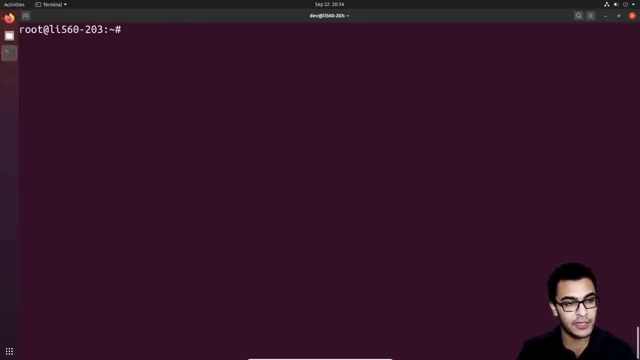 we. our first order of business, as I mentioned, is to log in or is to disable authentication, remote authentication with a root account, And to do this we need to. we need to take a look at the SSH or the open SSH daemon configuration file, Because the thing you have to understand about 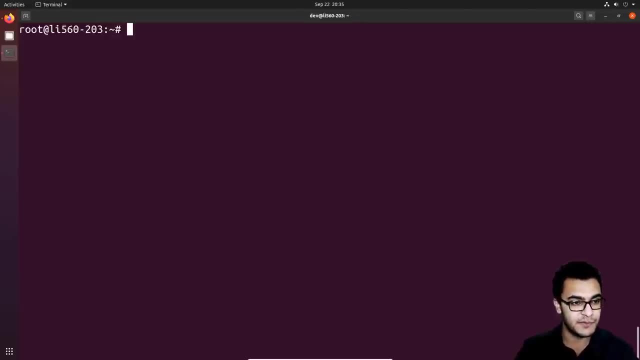 SSH. it is a client server based connection, which means there's the client and the server. this particular server is running open SSH server, So we need to configure the open SSH server settings. So we'll click. we'll use an editor. I'm using vim, you can use nano. So we want to go into. 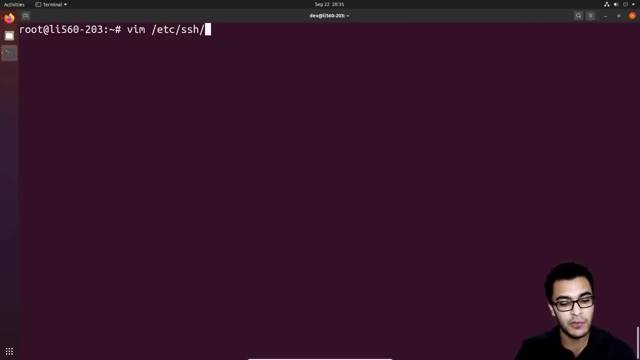 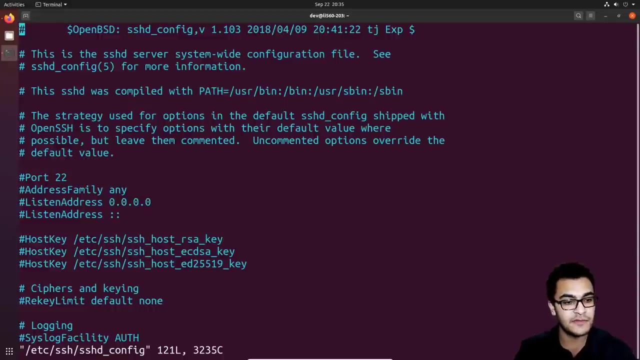 the Etsy directory, So Etsy SSH, And we're looking for SSH D. Now the reason we're looking for SSH D: the D represents the daemon, which essentially means the service or the server service, And we're looking at the SSH D configuration file. So we're just going to hit enter And this is the configuration. 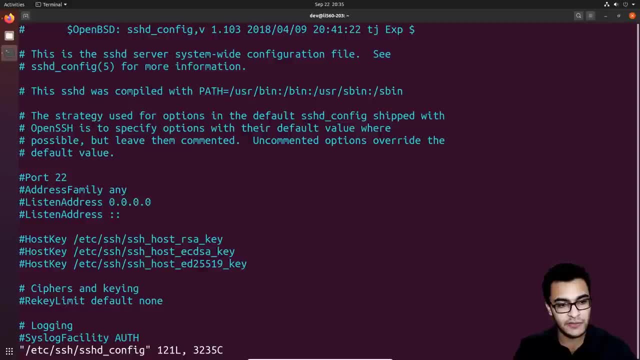 file over here. Now there's tons of options that you can change, And these options are not related, you know, only to security. they also pertain, or are also related, to things like networking. we can change the default port that the service is currently running on. that's also very helpful. 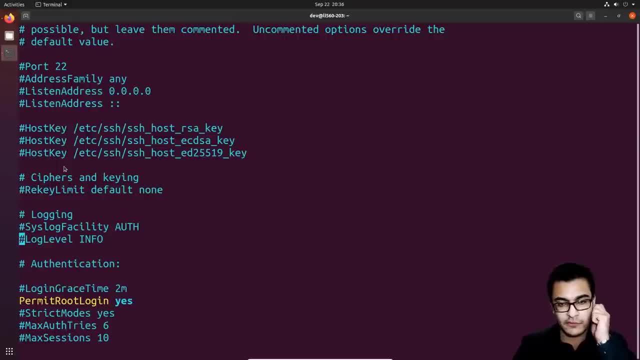 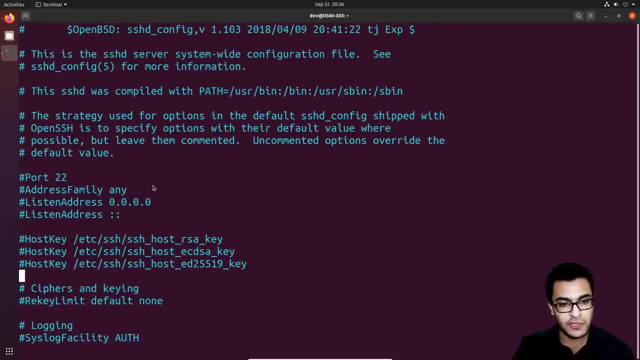 sometimes, And of course, there's tons of other options that we can change. Now, the option we're looking for is an option called permit root login. Now, the interesting thing you'll see about this file is the syntax that is used. Now we're going to go to the server. we're going to go to the 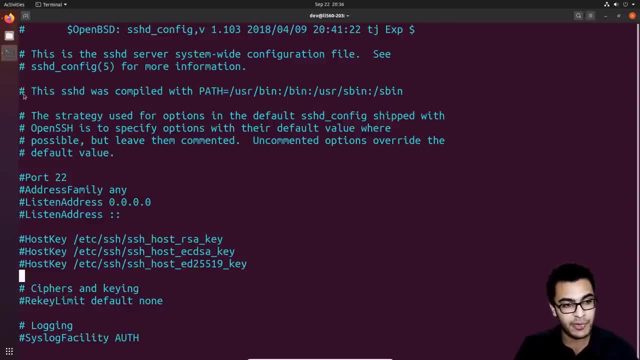 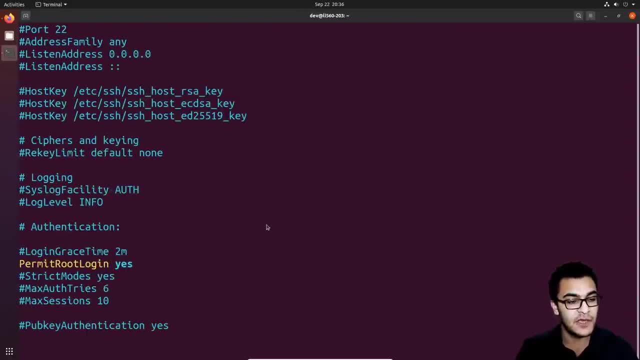 pound, that means that that line is currently active. In this case, all the lines with hashes or pound or the pound symbols means they're left to their default values And open open SSH will actually use that by default, So any custom options will will not have the pound or the the. 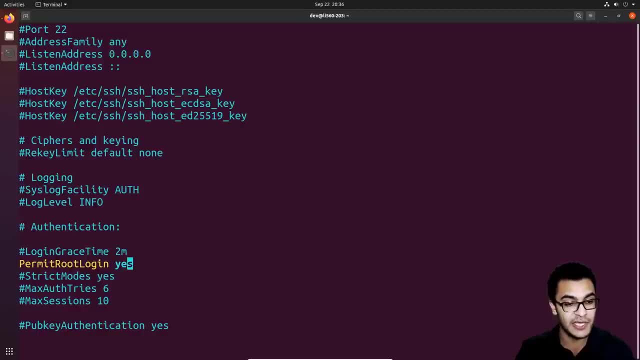 hash symbol. in this case, permit root login is set to Yes, we want to disable that, to know. Now note: this does not mean we cannot use the root user. that's something we'll be disabling in another video. This just means we cannot access the server via SSH using the root user. After this: 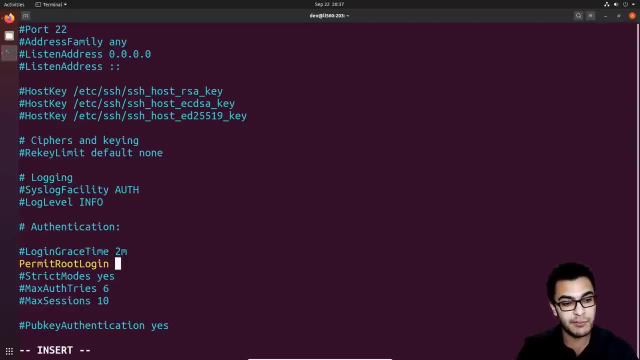 we'll only be able to access it using the dev user. So we'll say permit root login to know we want to say no to that And then to save this file. I'll just use W and Q to write and quit and we can. 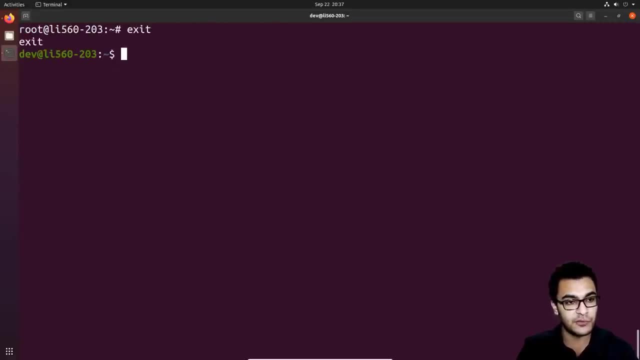 now quit. There, we are fantastic. So now I can just exit from the server. So I'll just exit from both users. There we are, And if I try and access the server using the root user again, you will see something interesting happen here And of course, I think I'll be able to authenticate. 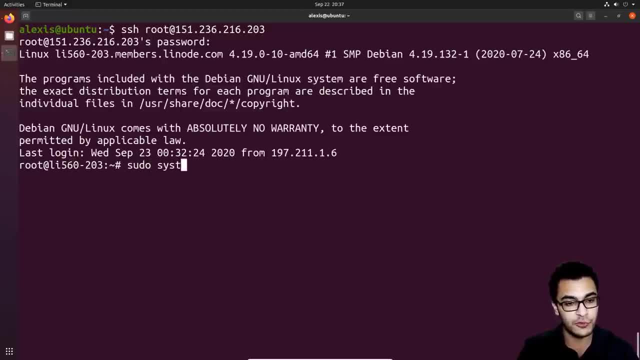 because I haven't restarted the service, So I'll just do that right now. So sudo system control, restart SSH and that will restart the service. And if I try and log in again now it's going to ask me for my password, And if I enter the password, 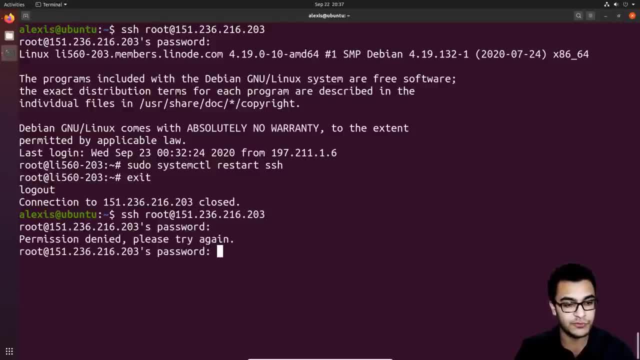 it's going to tell me I'm unable to authenticate, So we'll just wait there. we are permission denied. try again. And that doesn't necessarily mean that my- my password is incorrect or I've done anything wrong. It just means that I cannot log in to the root user with a password I cannot. authenticate with the root user via SSH And of course, you can see that that that option is explicitly defined within the configuration file. because it does. it does offer a reprieve in terms of security, because a lot of attackers will target the root account because it offers the lowest. 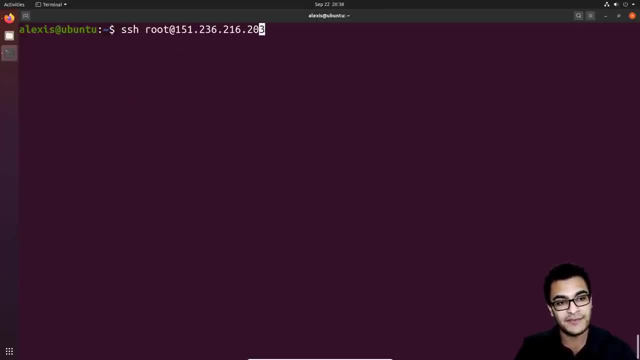 hanging fruit, Right. so that means we can only access the server via the dev user. Alright, so I'll open up the dev user right over here. Fantastic. So I'll specify the, I'll specify the password for the dev user and I have access and, of course, I can switch back into the root user. 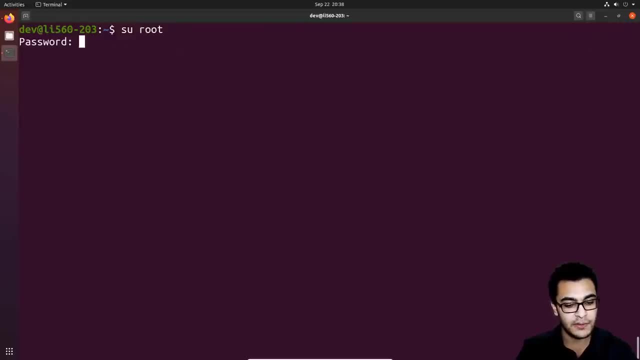 if I want to, by saying su root, And there we are Fantastic. So again I'm going to say su root, And there we are Fantastic. So again I'm going to say su root, And there we are Fantastic. So again. 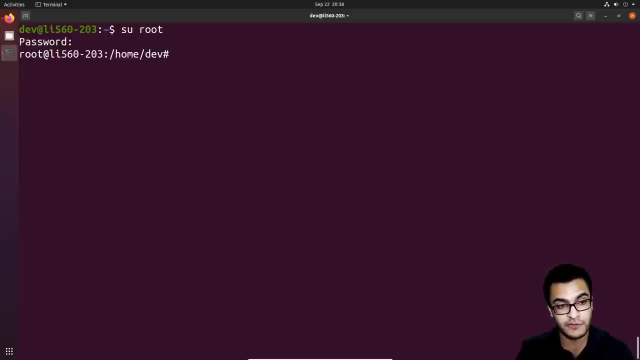 I can. I can always access the root user, But that's something we'll also want to be disabling, because the dev user, if compromised, can still in some way access the root account if they have the password. In most cases that's not going to be the case, But now we have to secure the dev user. 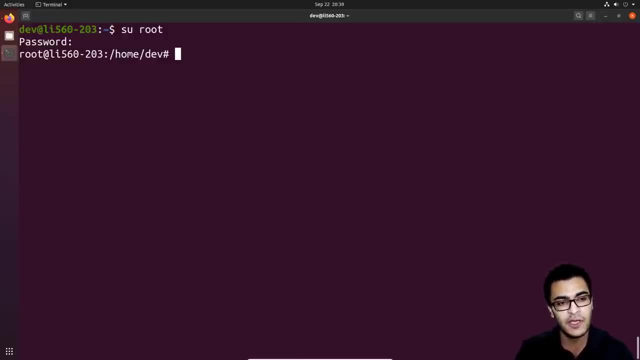 And the way we're going to be doing that is by using SSH keys. Now, as I said, we can set up SSH keys by default with a cloud provider likely known. however, that does it for the root user. we want to do this for the dev user, So we are slowly segregating. 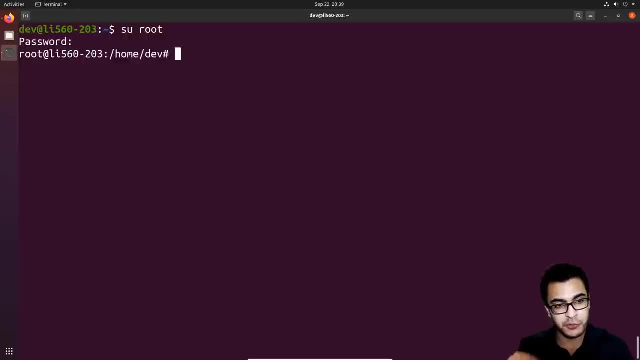 and lowering our, the, our security risk, because we're setting up users based on privilege And number two, we're also increasing the, the amount of authentication security in place. So, to get started, what we want to do is I'll open up a new tab on in my terminal here. 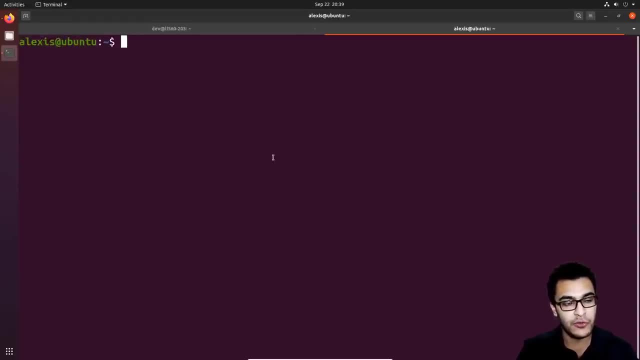 And we want to generate our SSH key Now. or you can generate your SSH key very, very simply on Linux by specifying SSH keygen. So if I say SSH keygen, like so you can see it gives me the ability to generate a key. So 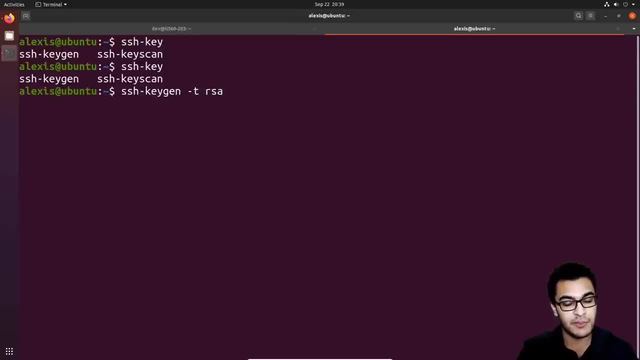 a sage key, then I can then specify T RSA. that is the, the algorithm that is being used And on Windows you can do it. you can also generate your SSH keys using using putty, if you want, and I'm going to enter And it's going to tell us it's generating the public, private RSA. 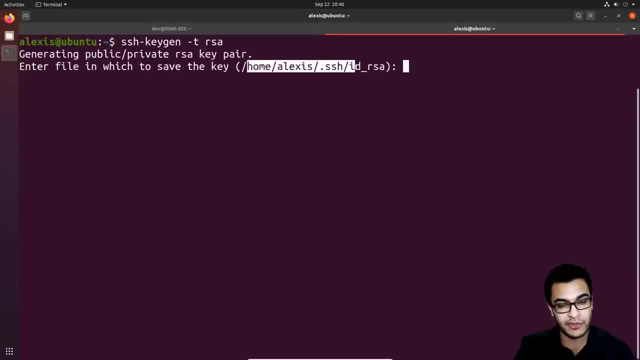 key pair and it's going to save it into the default home directory under SSH Here. in most cases you just want to leave that as it is, So I'm just going to enter and it's going to tell me it already exists And I'm going to overwrite this for a very important reason. on it: enter. 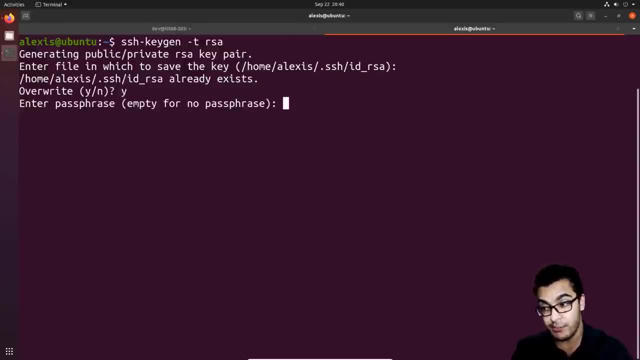 Now, SSH keys also allow you to specify a passphrase. This is like two factor authentication, because in addition to SSH keys, you can also secure them with a password. So if someone gets a hold of your SSH key, they'll not be able to authenticate without that particular passphrase. 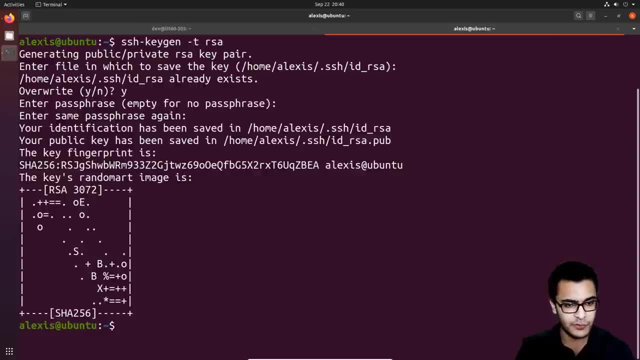 In my case, I'm not going to enter a passphrase, So I'm just going to enter right and your, your. your keys are going to be stored within your home, your home directory, under SSH, And the file is going to be called ID RSA. That's your private key, And you have ID RSA dot pub, which means 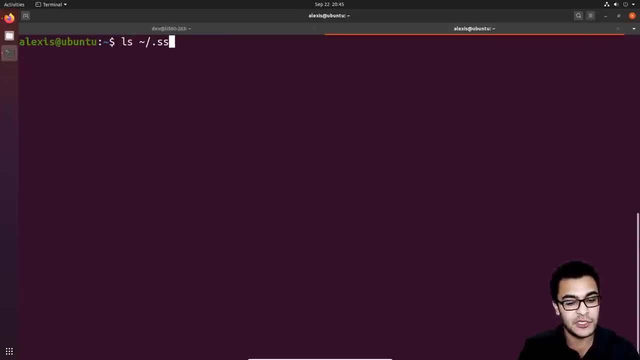 public key that we can list out the contents of my SSH directory here. So SSH, and if I listed, you can see we have the private key. this is what we want to keep securely And we have the public key. Now, of course, when we talk about the- the public, as I said, 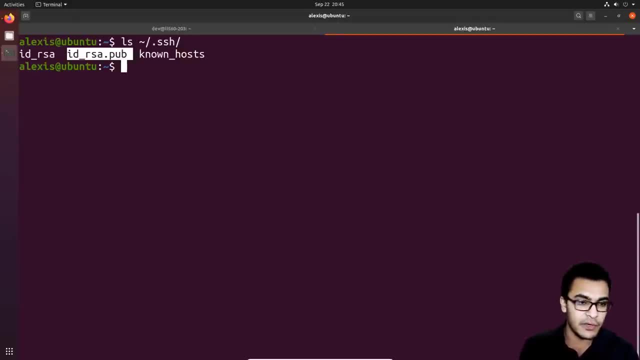 we need to copy this onto the server. So how do we do this? Well, we can. we can copy it manually. However, much easier way of doing it is through a utility called SSH copy ID. So we say SSH copy ID, And then we specify the user that we want to authenticate as so dev at, and then I paste in the 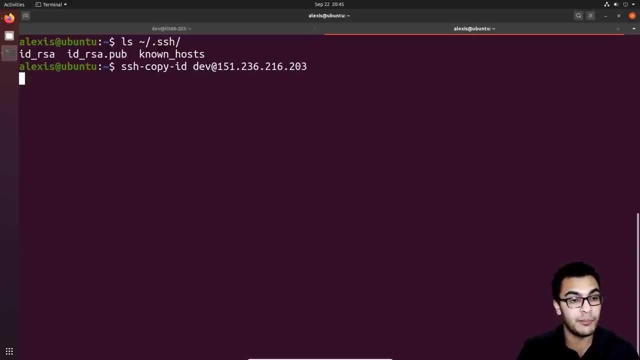 IP of the server And I hit enter And that's going to copy our public key to the server. So we're just going to wait for that to prompt us to authenticate with the password. So it's going to send our password for the dev user. So there we are. it's going to now tell us. 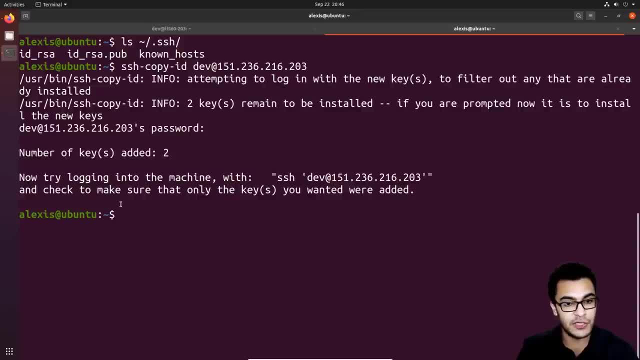 the number of keys added is two. right, So we've added two keys. here And there we are. So we've added our key, And that means we can now authenticate to the. we can authenticate to the server without entering a password for the dev user. That's only for us, However, a password based 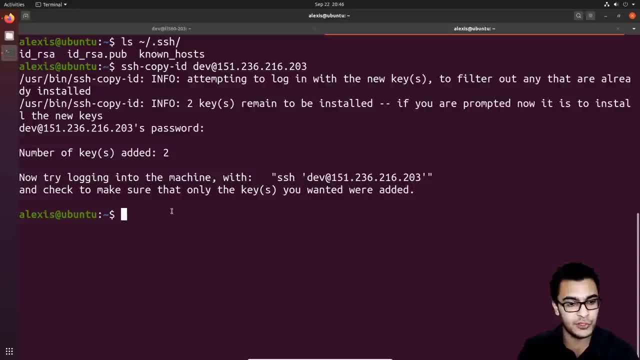 indication is still available, So I'll just explain this to you shortly. So if I try and log in to the SSH, to the server, via SSH, using the dev user, you'll see that I'll be able to log in without entering a password. So I'll hit enter. it's going to use my private key And again. 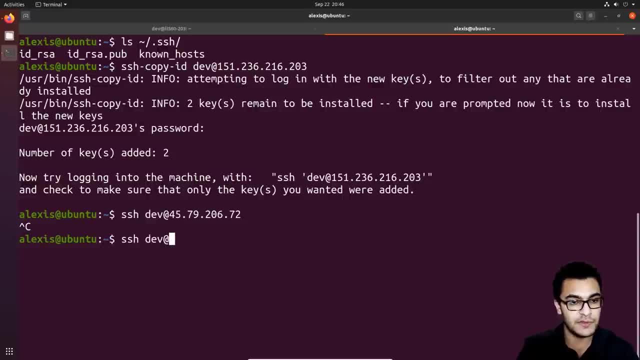 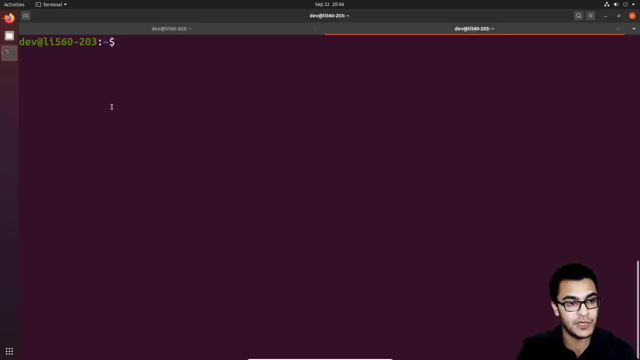 we'll just sorry, that is an incorrect IP. let me just paste in the correct one, which is this one right over here. If I just paste that in here and you can see, I'll now be able to log in without entering any password. There we are. I'm now logged in as dev at the Linode instance. 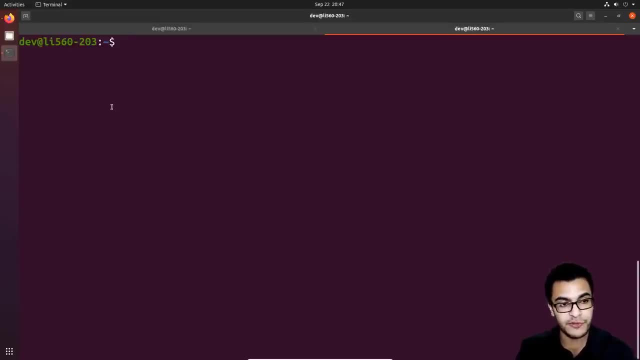 right over here. So I didn't have to enter any password, Although password based authentication is still set up. Now, if I try and authenticate using another system, like my Windows system with putty, and I'll just open up Linode and copy the IP there and I try and log in, let's open up putty. 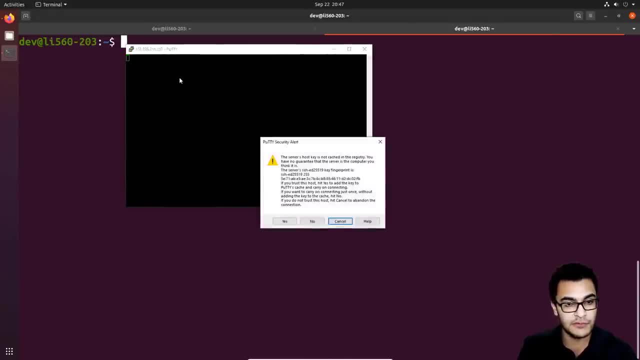 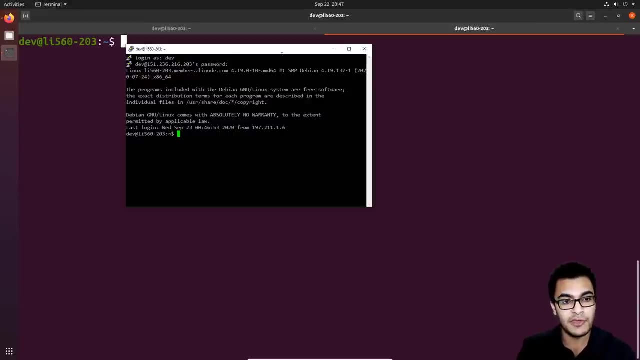 again Like. so you can see that it still is going to ask me for my password. So I'll say you log in for my password And I can still log in regardless of whether I've set up an SSH key. we need to remedy this. The way we remedy this is by disabling password logins or disabling. 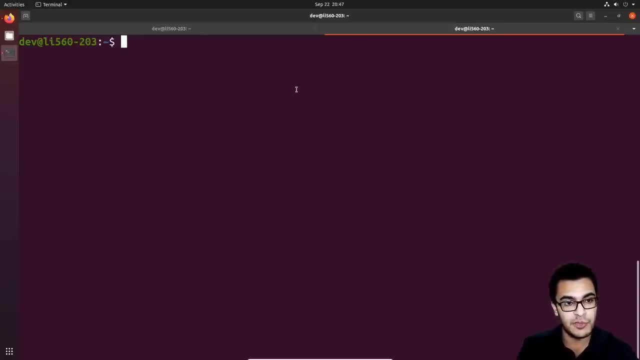 password based authentication. So what I'm going to do is I'm just going to minimize that and I'll switch into the root user. So I'll say su, root And it's gonna ask me for my root password. There we are And we'll go back into the SSH D configuration file. So 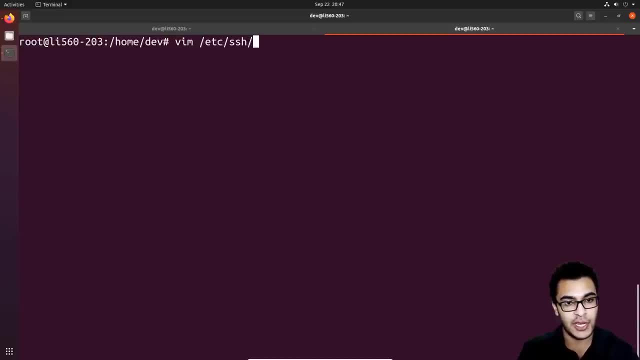 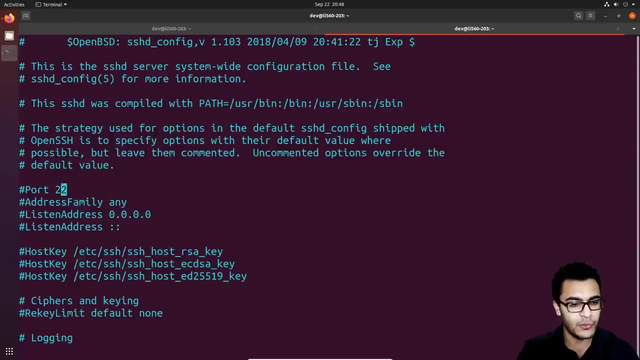 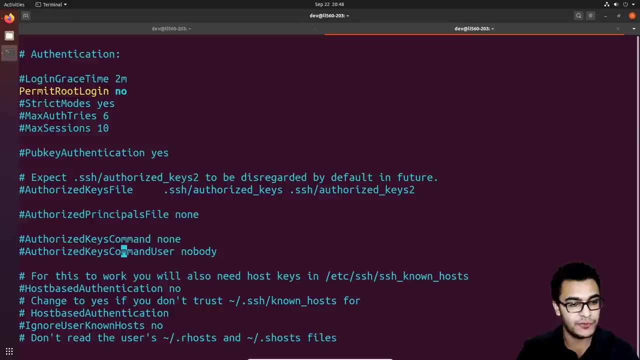 we're looking into the Etsy, SSH and SS HD configuration file And we want to go. we want to go all the way to the bottom here, right over. it should be over here Under authentication. we have changed permit root login to know And we just want to go slightly to the. 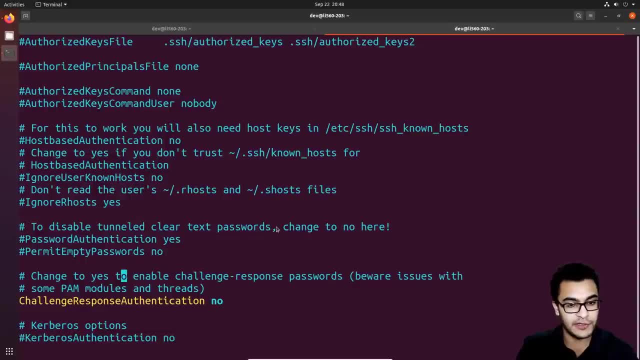 bottom here on under disabled tunneled clear text password. So to disable tunnel clear text passwords. we're going to change to know here. So for password authentication we want to disable this. So we again we'll just get rid of the, the pound or the hash symbol And we're going to set the 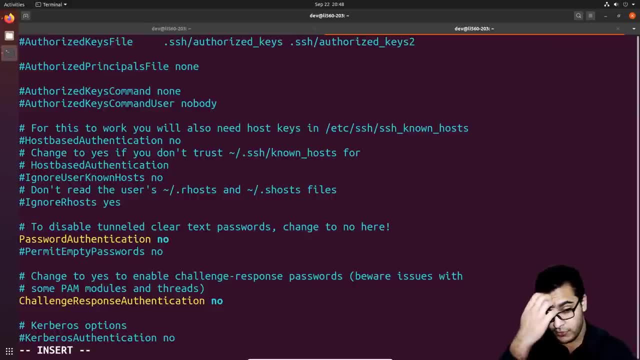 option to know right, So we'll set that to know. Now, what this means is that under no circumstance are we going to be able to access this server using passwords. the only way we're going to be accessing this server is through our SSH keys. So that's something you want to take into. 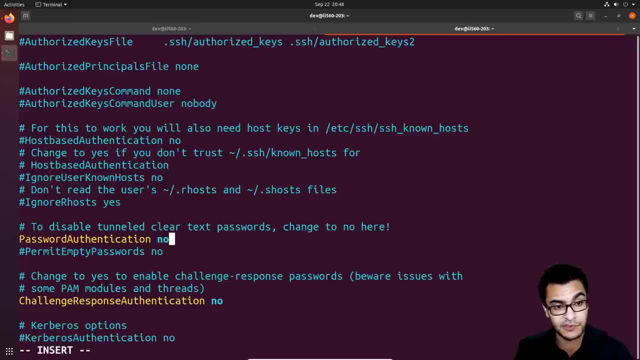 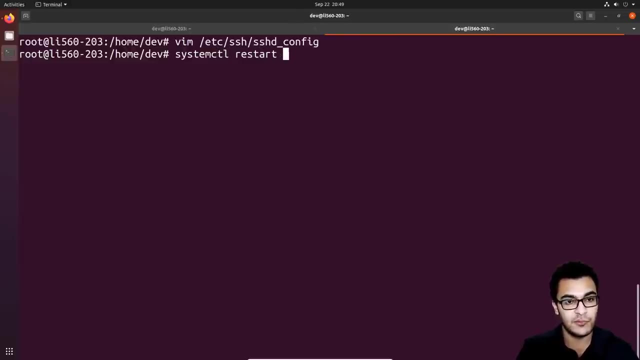 consideration. activate this particular option or this particular setting. make sure you have the SSH key available, because there'll be no way you'll be able to get access to this fire SSH then. So I'll write in, I'll write the changes and save it, And again, in this case, I'll just restart SSH. So system. 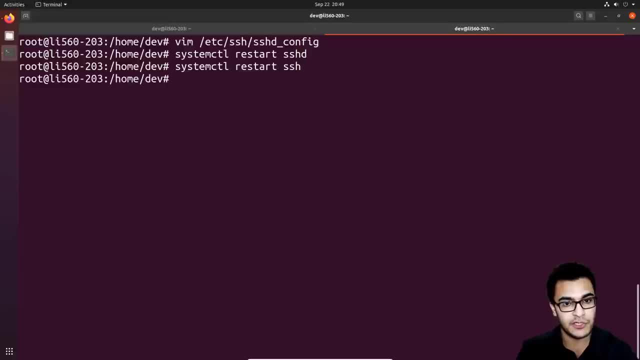 control, restart SSH. sorry, SSH like so, And if I now exit or I log out again on this system, I'll be able to log in without the password because I have the SSH key And I can then share this SSH key with the development team and they'll be able to log in using the SSH key. 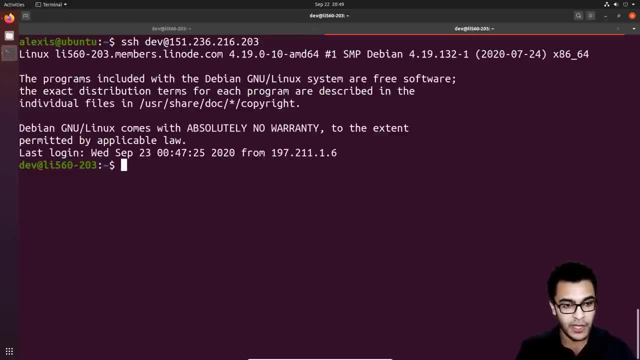 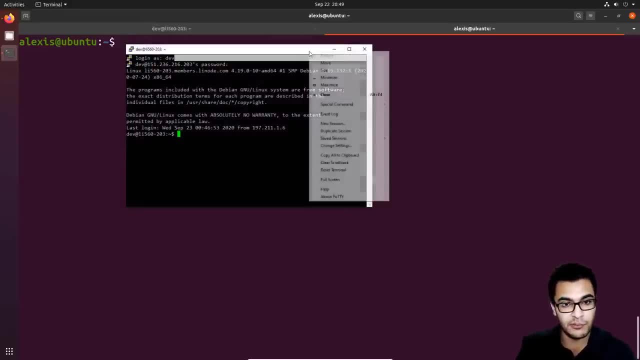 So if I hit enter, you'll be able to see there we are. I have access. I still have access here, However, if I go on over to my Windows system and I try and log in using putty. So what I'll do is: 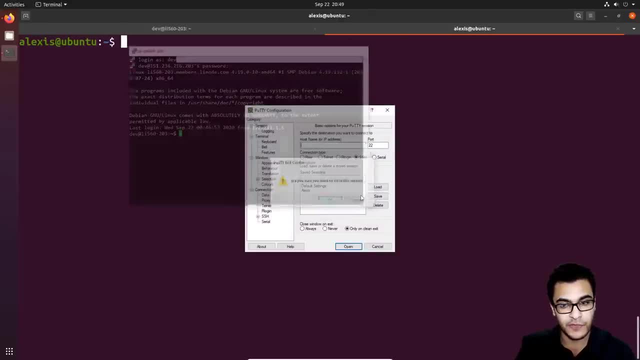 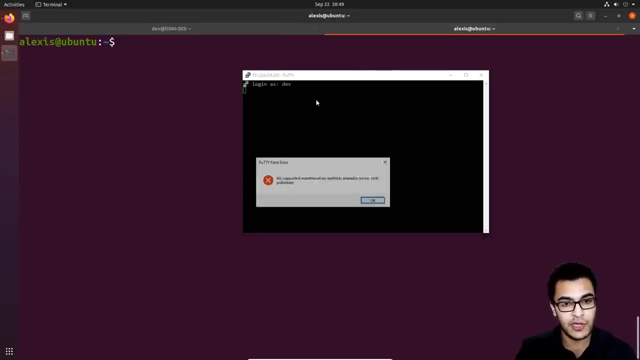 I'll just open up a new session here, I'll close that one And I'll just copy the IP one more time here, just to make sure I have the right one. And I'll open up putty, Let me just load my profile. hit open. You can all see. if I try and say login as dev, it's going to give me an error. 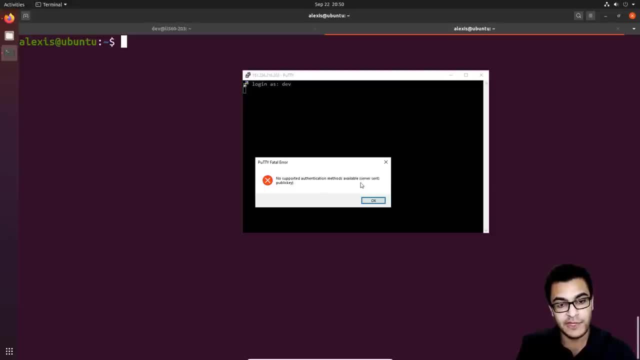 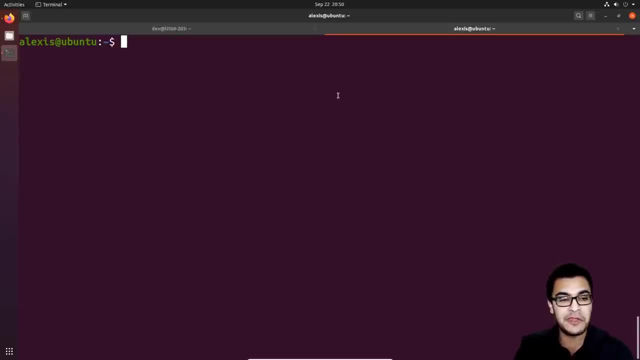 telling me no supported authentication methods available. server sent public key. So again that means that now on this server there's no way we are authenticating with with any password of any kind, regardless of the user. So again, we've disabled the root user logins, which is: 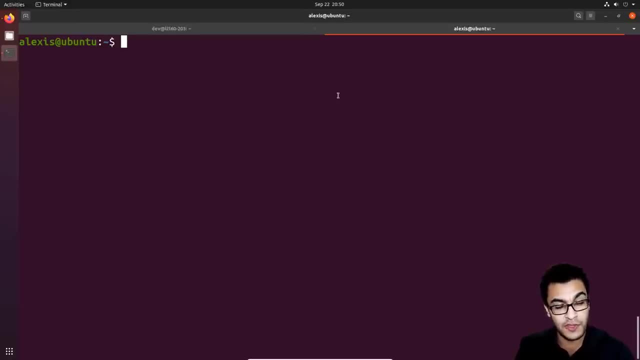 very important. Number two: we've set up and secured the other user account, which is the dev user. The only way anyone is logging on to it now is through the SSH key And, of course, as I said, the SSH key is going to be under your home directory in SSH, And it's it's the file that 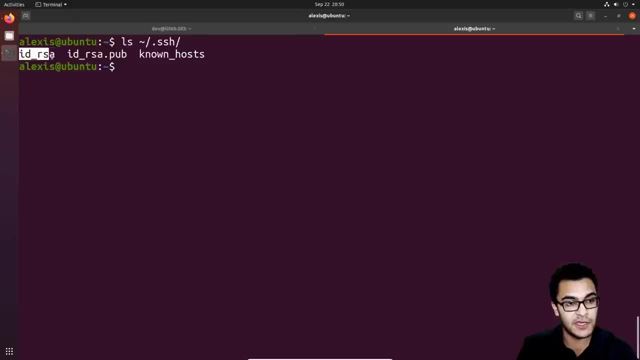 is in that we're referring to is the ID RSA key right over here. So this is the file you want to share with the development team And again they can then use it to log in. However, as I mentioned, it's very important to take into consideration the fact that you want to keep the private key.